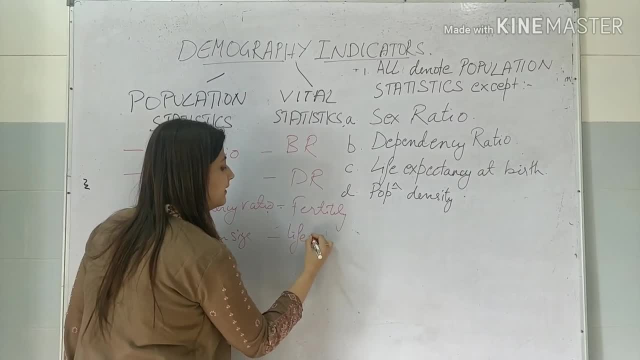 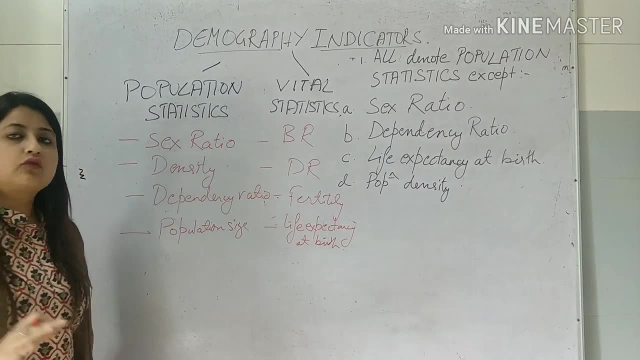 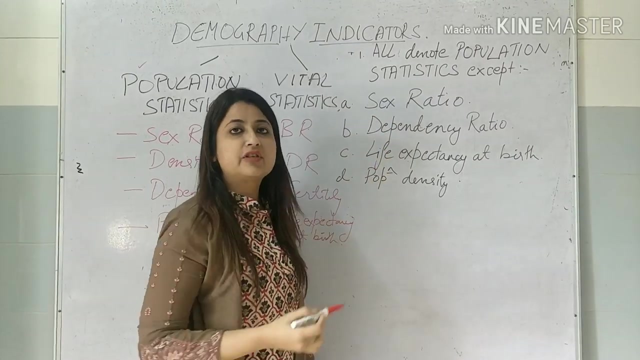 fertility. Okay, You also study the life expectancy and birth. Now, what I just told you, this could be a potential MCQ question that I have put down here for you. The question could be all remote population sizes. So what are the population sizes? What are the population? 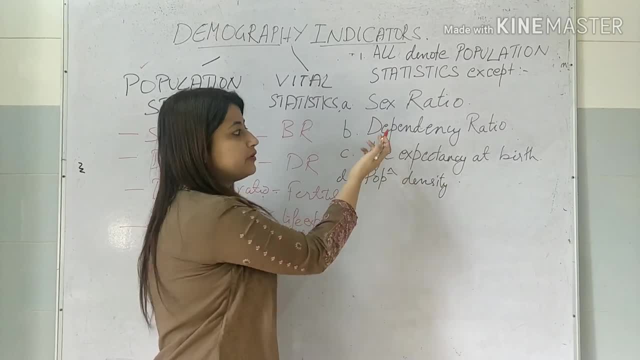 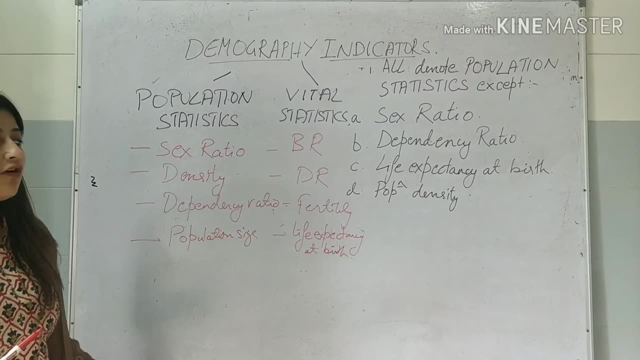 statistics. Are there any population statistics Except option A- sex ratio, option B- dependency ratio, option C- life expectancy at birth or D- population density? So from this chart it's very obvious that your answer is C Rest, sex ratio, dependency ratio and population. 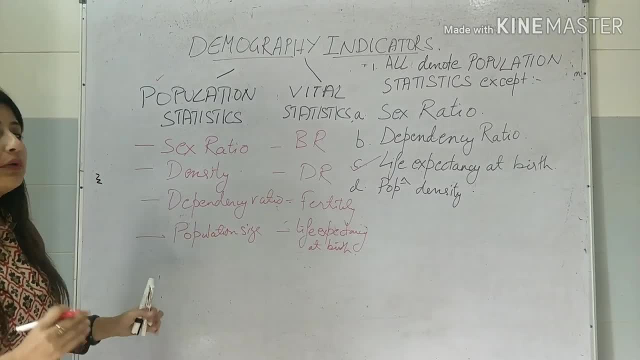 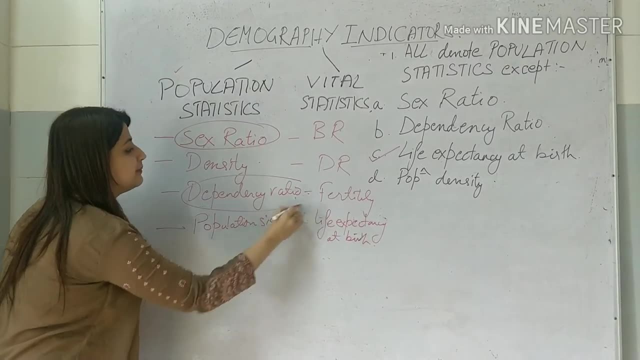 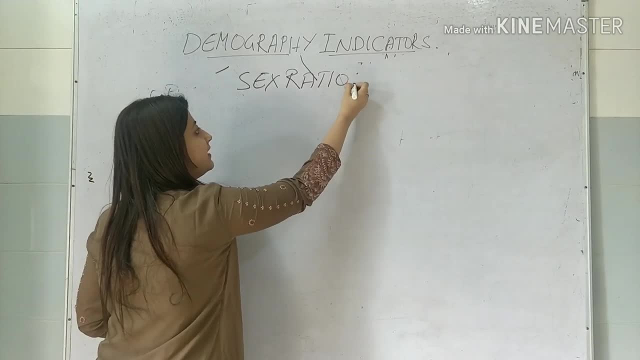 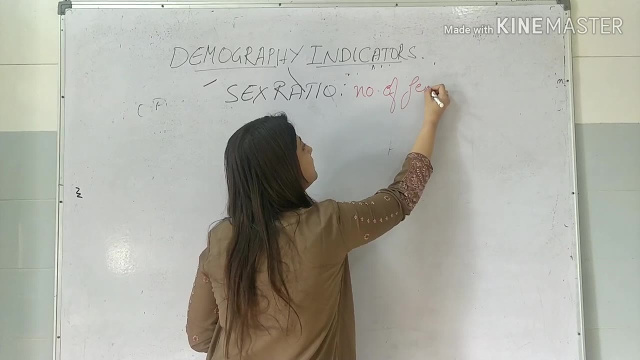 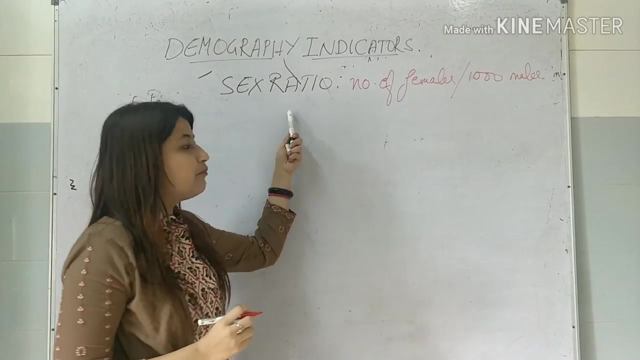 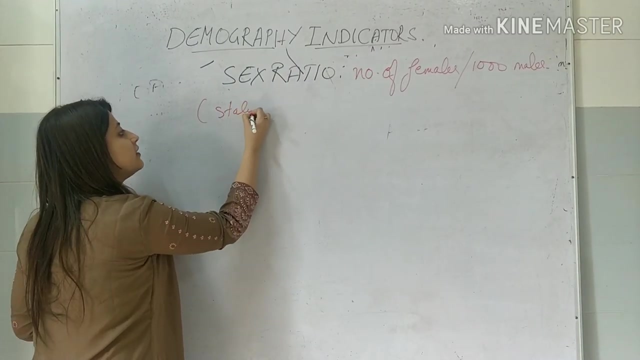 ratio. What is sex ratio? Nothing, but it is. the definition is number of females per thousand males. What is the importance of this indicator? This is the only indicator that highlights the status of a woman in a community or in a society. Now, since we are studying sex, 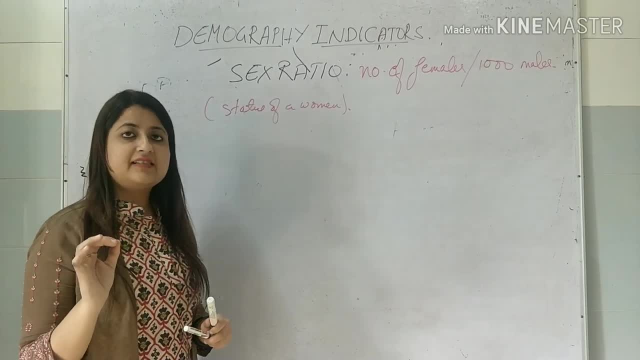 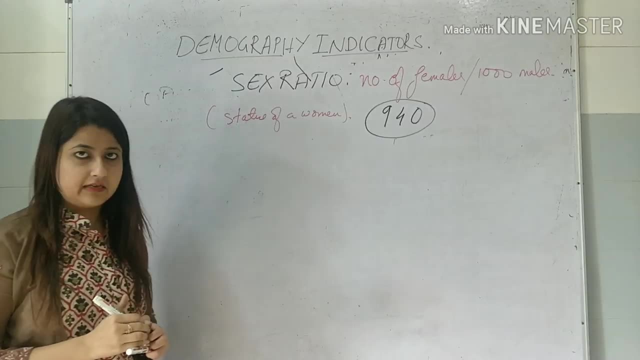 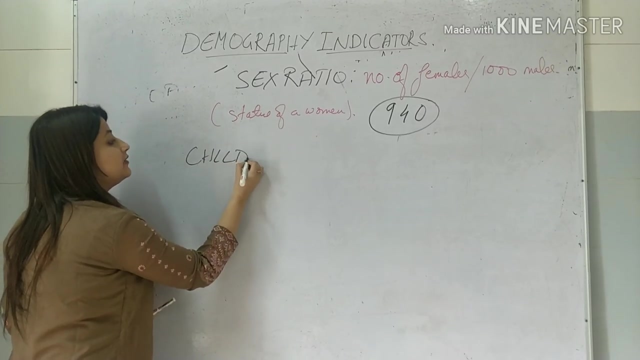 ratio. what is the current sex ratio of India As per census 2011,? the current sex ratio for India is 940.. This could also be asked in a MCC Moving ahead. there is another sex ratio that you must know. that is child sex ratio. Either of these two are the same. 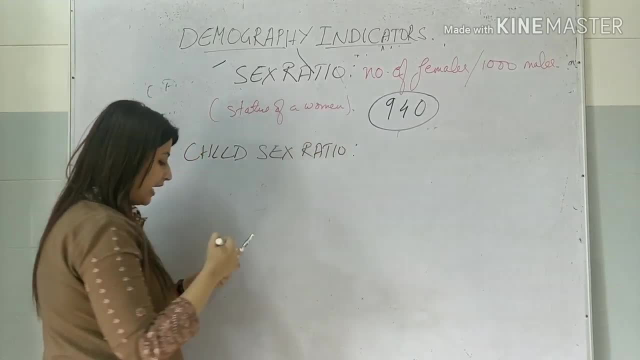 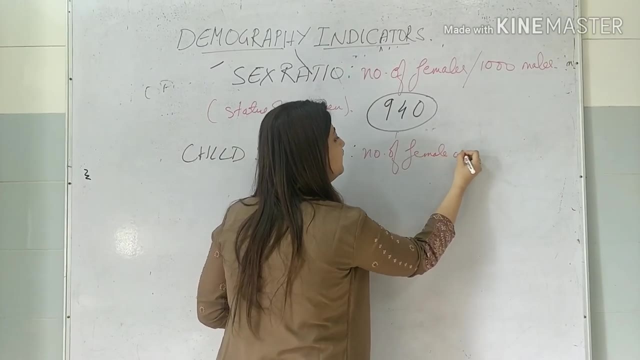 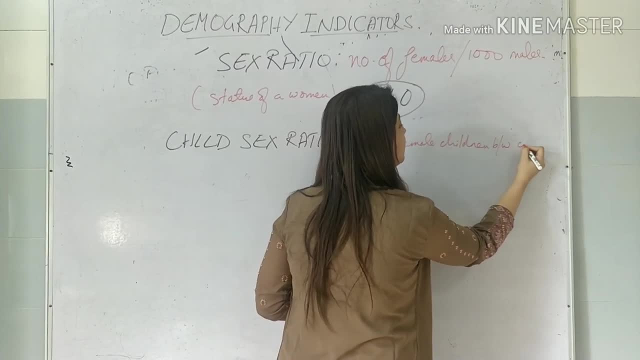 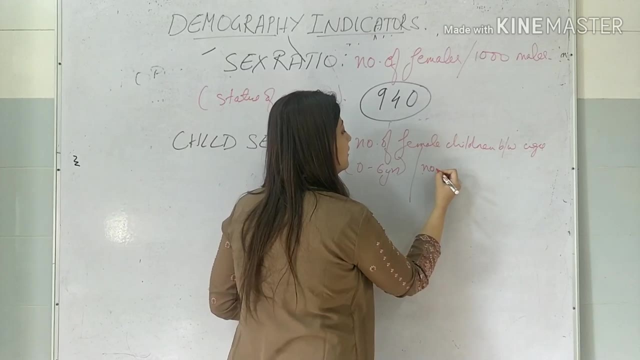 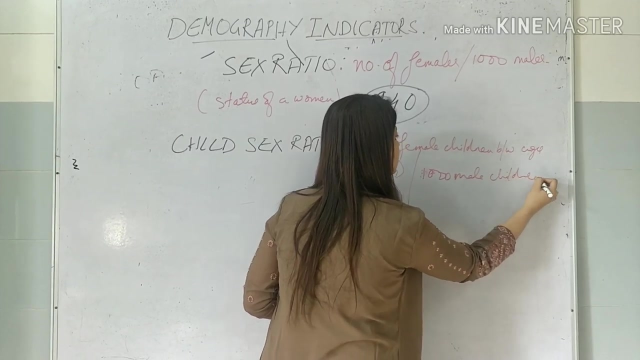 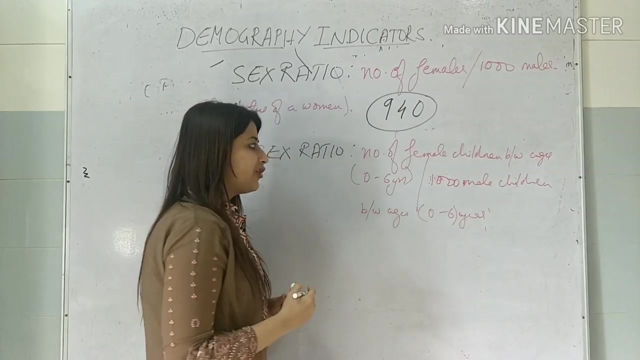 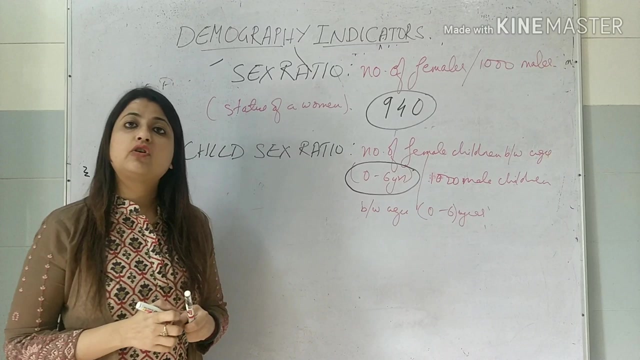 between ages 0 to 6 years to per thousand male children between ages 9 to 10 years. between ages 0 to 6 years. What is the important thing here, which could be asked as a question, is that it includes children between 0 to 6 years. Now, current child sex ratio as per. 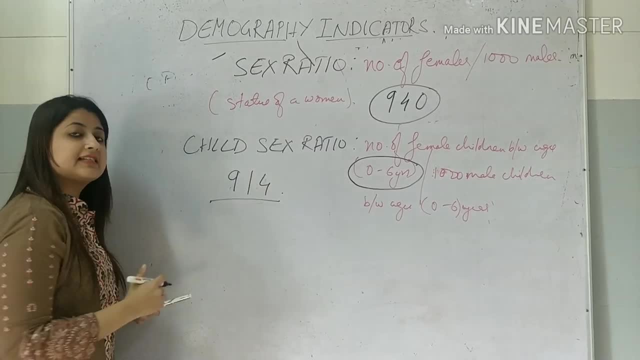 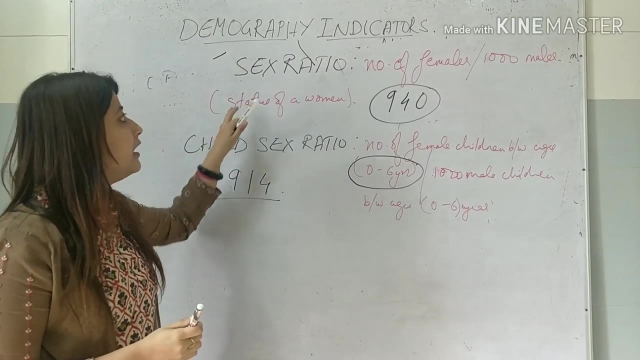 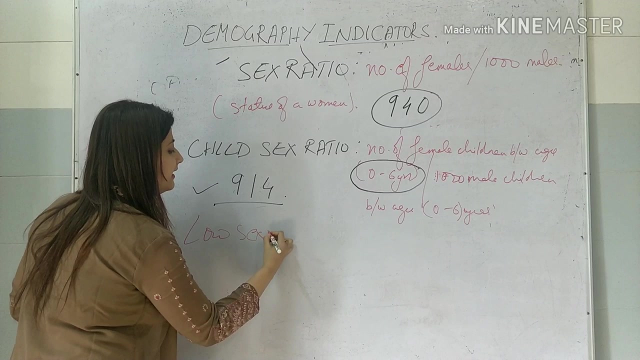 census 2011 is 940.. It has hit an all time low of 940.. So the question that could be asked in the viva examination is that: what does a low child sex ratio indicate, Or what does low sex ratio indicate? So here you can definitely see: a low sex ratio indicates gender. 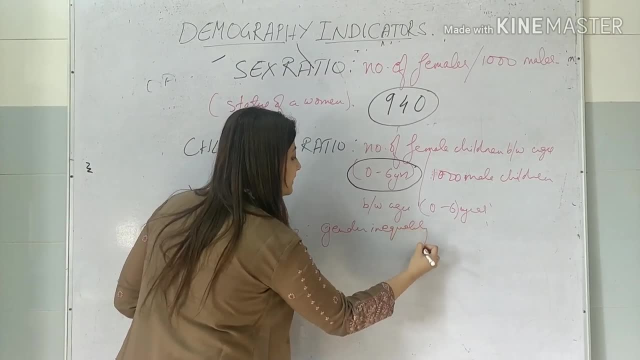 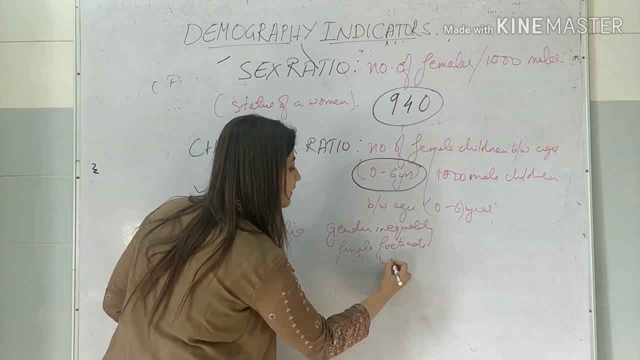 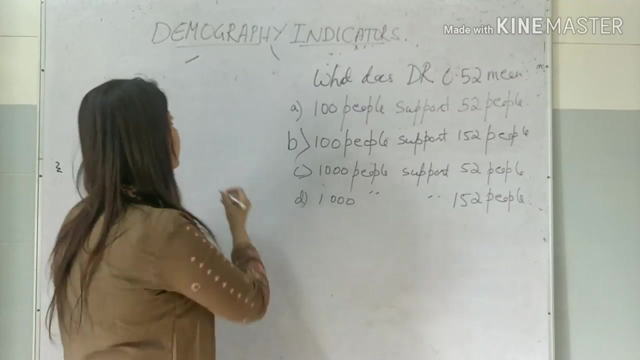 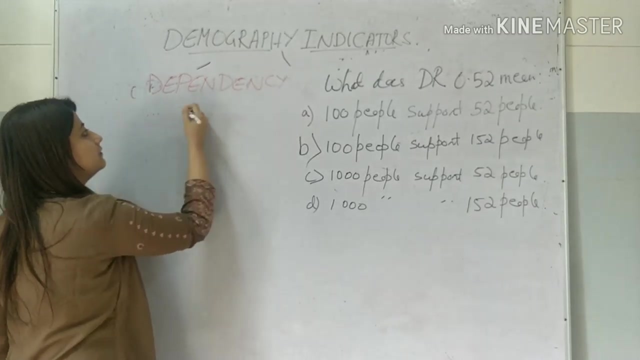 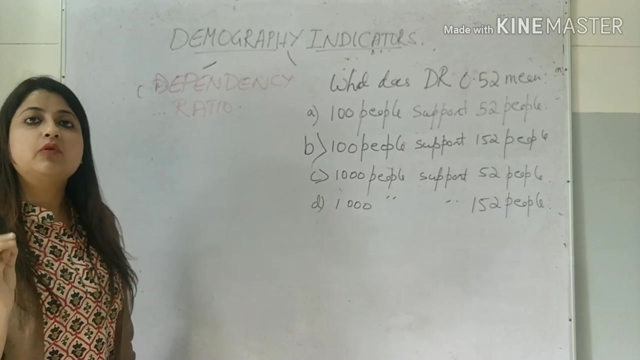 inequality. Also, it indicates female feticide, Or you can say it indicates female infanticide. Next, we will be discussing the underage. So underage is another important demographic indicator, which is dependency ratio. Now, as you have seen this word, there is a term dependency. That means there are some who are dependent. 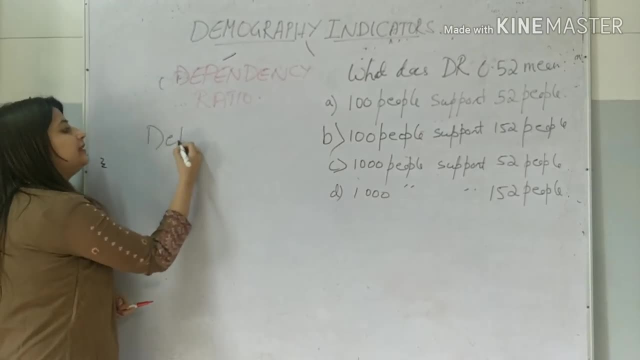 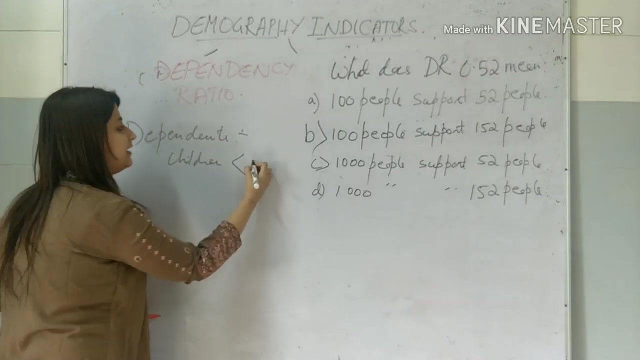 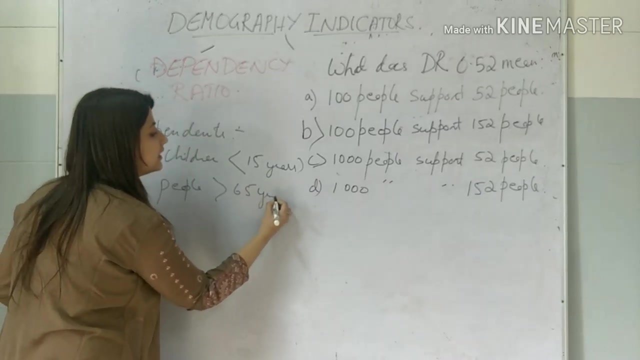 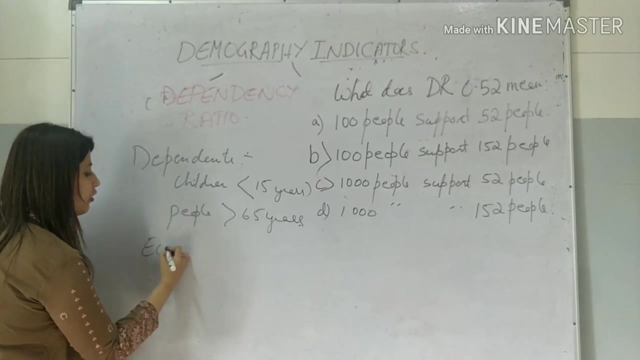 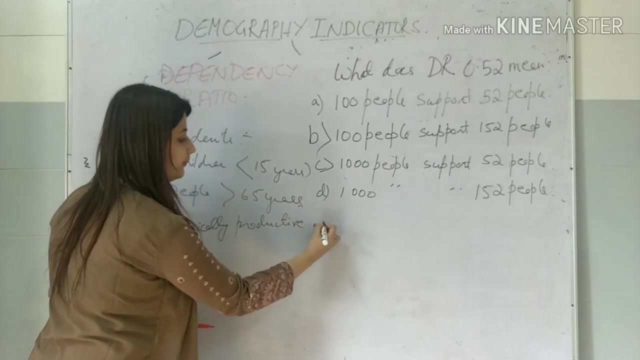 So who are the dependents in the society? The dependents are children who are below 15 years of age And people who are above 65 years of age. That means if there are dependents, there are some who are not dependent, which is the economically productive age group, So that economically, 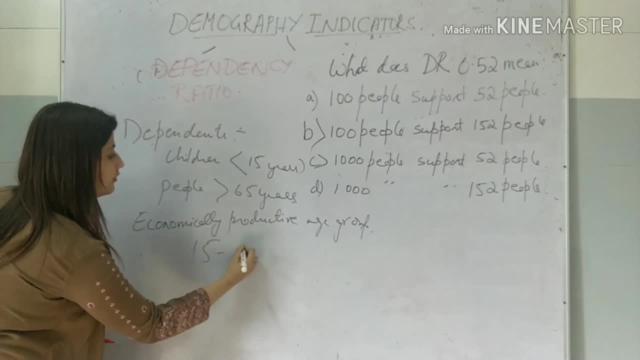 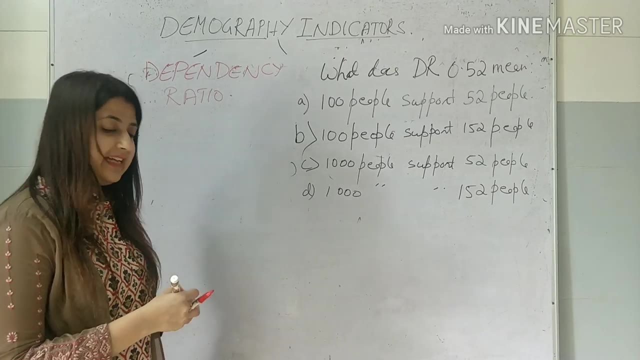 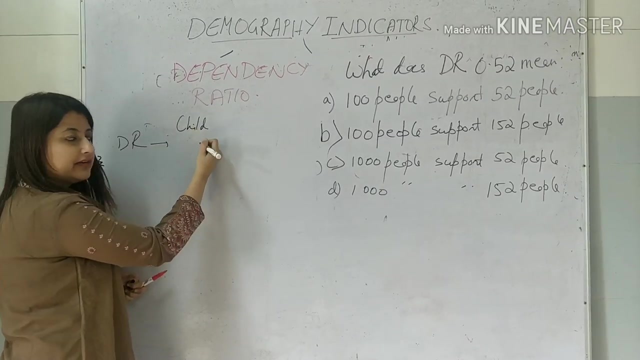 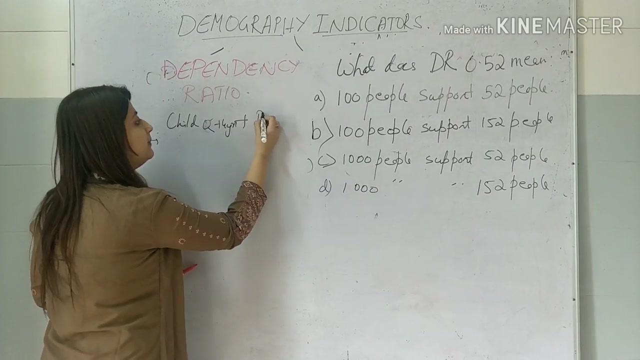 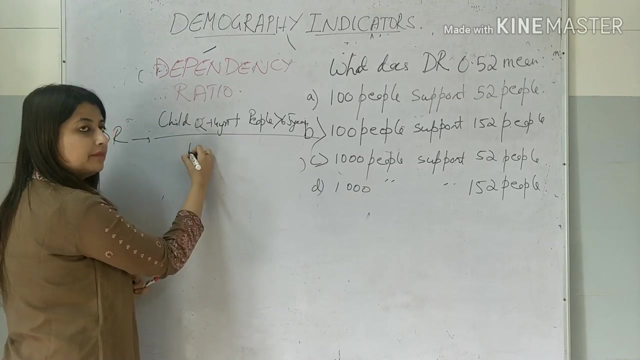 productive age group becomes 15 to 64 years. Okay, Okay, Now what is the dependency ratio? The dependency ratio? it is nothing but the ratio of combined age group- Children 0 to 14 years of age, plus people more than 65 years of age- upon people. 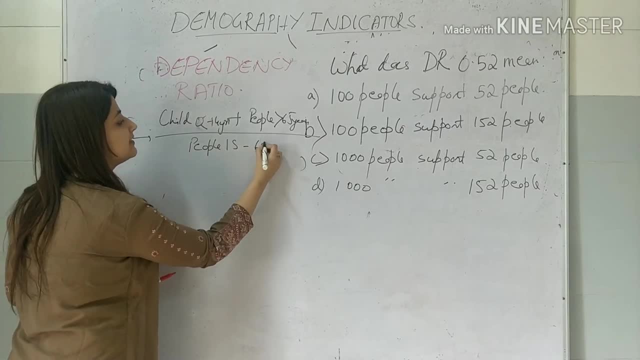 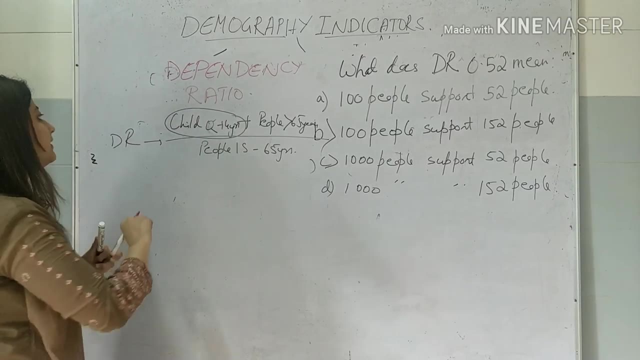 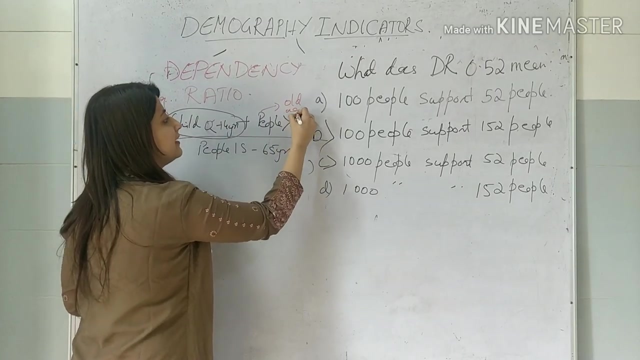 between 15 to 65 years. This is your dependency ratio. How is this ratio So? in this you can see that one is the young age dependency ratio and the other is the old age dependency ratio. Now you will be amazed to know that, because of improvement, in family planning services. there is a decline in fertility. So the young age dependency ratio is gradually decreasing or declining and the old age dependency ratio is increasing. Why? Because of increase in life expectancy, because of increase in longevity, due to improvement.